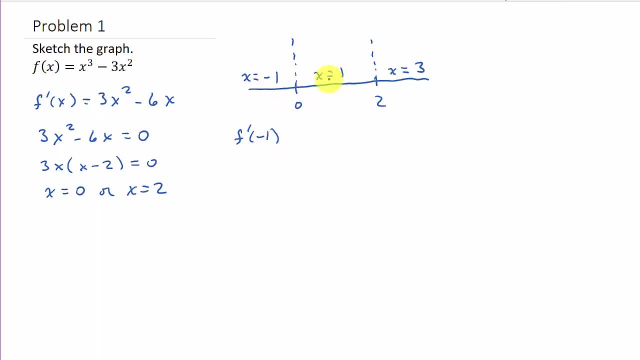 We have to evaluate the derivative at each one of these x values. Now, when we take the negative one and we plug it into the derivative, we can take the negative one and we can plug it into here. Okay, that's fine, But this function right here it's the same thing as this one. 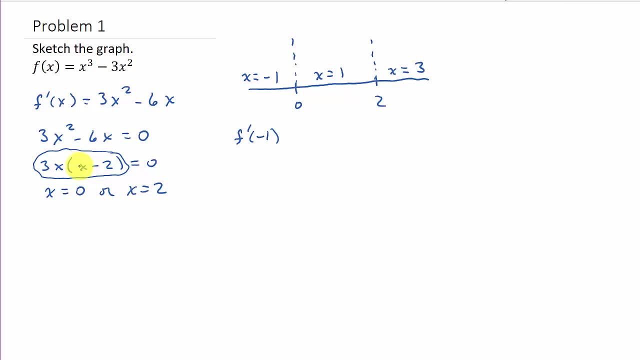 It's just this is factored. Okay, but they're the same thing. So, yes, you can take the negative one and plug it in and 3 times negative 1 is negative 3, and negative 1 minus 2 is negative. 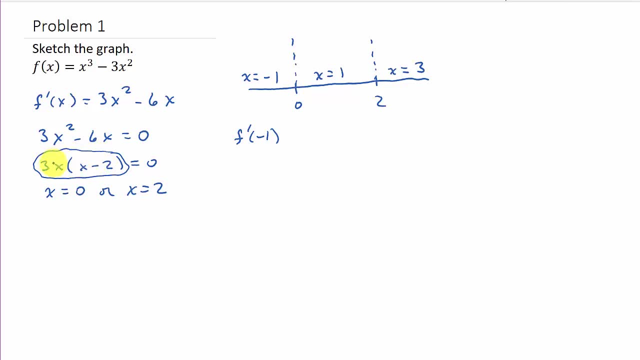 3. 3 and negative 3 times. I'm sorry, yeah, negative 3 times negative. 3 is positive 9, but you don't have to go that far with it. all we really care about is when we plug this value in for x into. 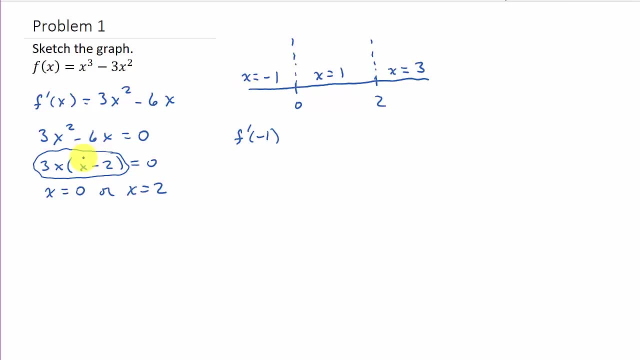 the derivative. is it positive or negative, that's all we care about. so if you look at this, this negative 1, if we plug it into here, you can see 3 times negative. 1 is negative. and then if we plug the negative 1 in here, negative 1 minus 2 is negative. so this is a negative times a negative. 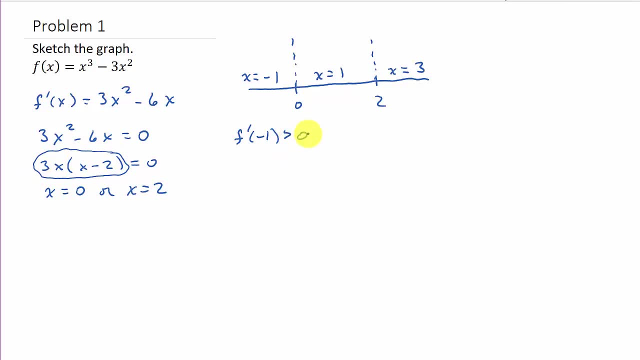 is positive and that's all we care about. we don't care about what the exact value is, all right. so since we plug the negative 1 into here and we got a positive as an answer, that means on this interval here, this function is increasing. all right, and then 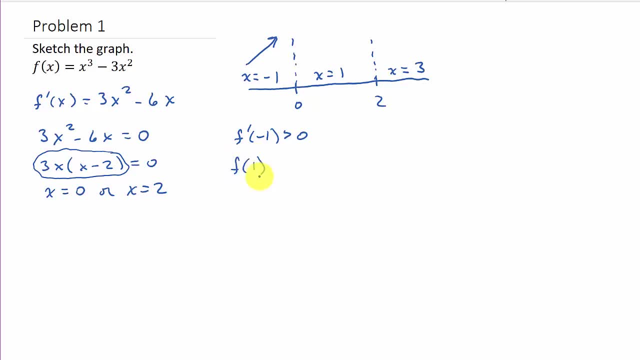 we're going to plug in the 1. so if I plug a 1 in for x 3 times 1 is positive, 1 minus 2 is negative. so a negative times a positive is negative, and so that means on this interval it's decreasing. and then we do- I'm sorry, and this should be f prime- and then we do f prime of 3, so 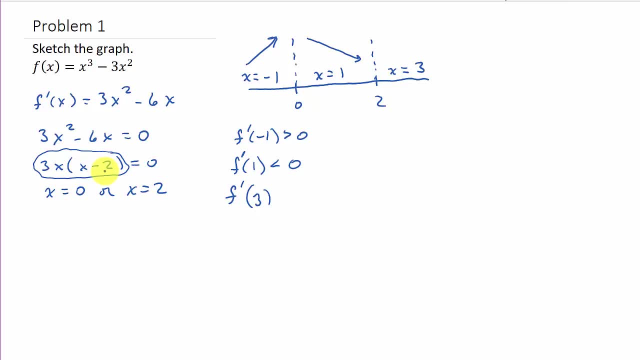 3 times 3 is positive. 3 minus 2 is positive. a positive times a positive is positive. so that means it's increasing there. so that means we have: this is decreasing from 0 to 2 and it's increasing from negative infinity to 0 and 2 to infinity. 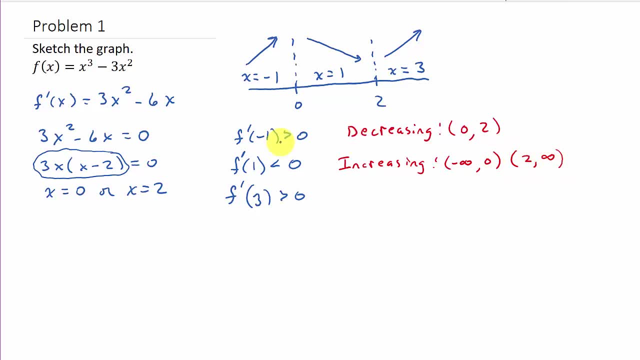 now on here, I can write these in different colors and the the the stuff that I need to graph my function. that's what I'm doing. I'm gonna write it in different colors. what I would recommend is you put like a star beside the things that you need. 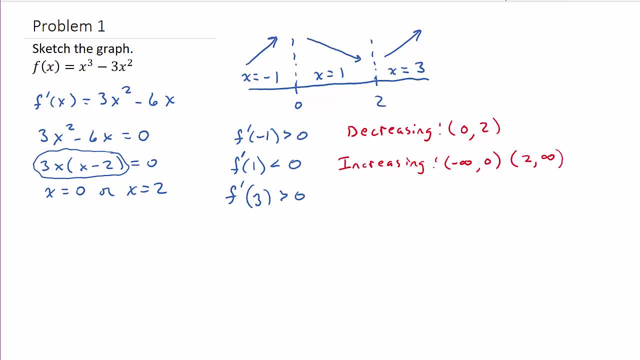 and this is one of the things we need: where is it increasing and where is it decreasing? all right, now let's find any local maximum or minimum, or relative maximum or minimum values. ok, so it's easy to find that once we find where the function is increasing. 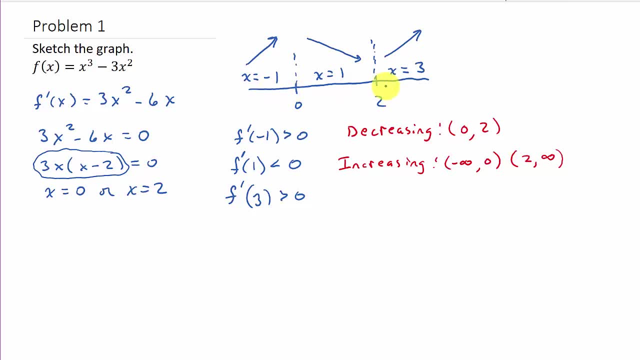 and decreasing. so if we look at this, where we found where it's increasing and decreasing, you see here on this interval how it's increasing and then at 0 it starts to decrease. so that means it's x equals 0. we have a local maximum and then look. 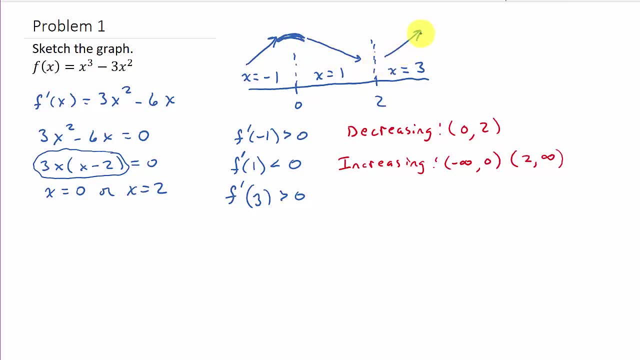 here it's decreasing and then at 2 it starts increasing again. so that means we have a local minimum right here. all right, so we have a local minimum at where, at X equal 2. you see that. alright, now your local maximum and minimum values. those are point coordinates on the graph. so you can see here we have an x. 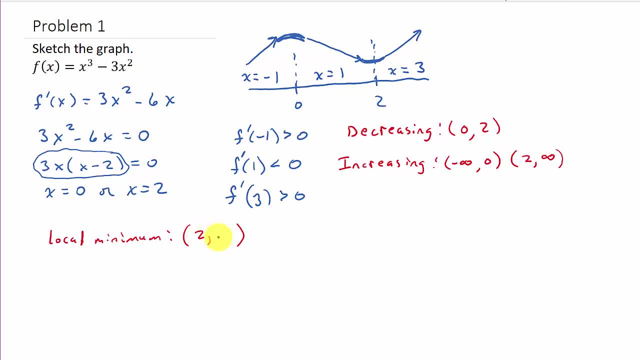 coordinate. well, now we need the Y coordinate well. how do you find that? this is where a lot of students get confused. they don't know where to plug the two in. a lot of them will plug it back into the derivative- all right, but remember you're looking. 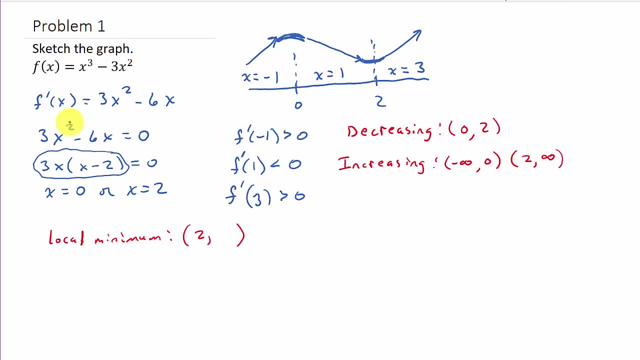 for a point coordinate. so if you have an X coordinate of the point, how do you find the Y coordinate? well, you plug it back into the original function, right? you take the X value, plug it in for X into the original function and then that gives you your y coordinate. so I have F. let's do that in a different color. so 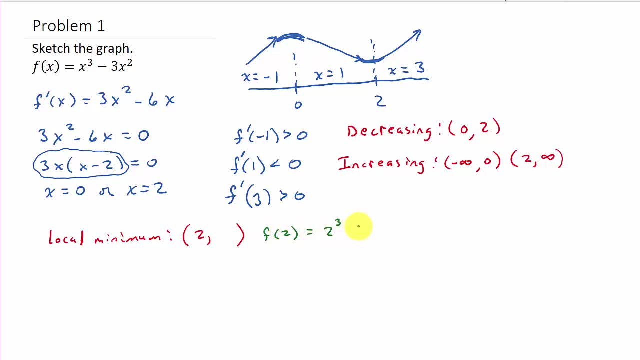 I've got: F of 2 is equal2, 3 times 2 squared. and for that we've got let's see 8 minus ths times 1. If we plug that back into the derivative of the x's, as we can see, then that gives you the Y coordinate. Here's K squared. and then if we let the y coordinate, 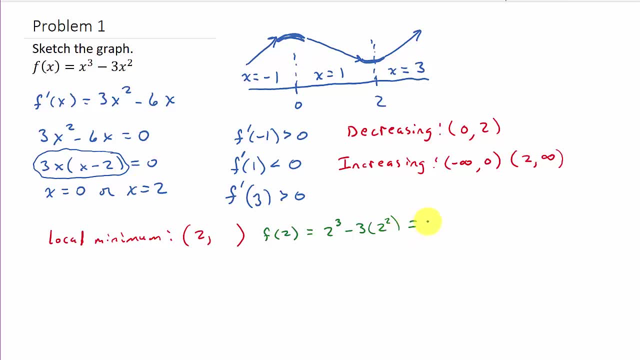 connected. we you plug in the y coordinates and we plug that back into the original. minus 12 is negative 4, okay, and so the y-coordinate is negative 4, and then we've got a local maximum at x equals 0, say our local maximum here. so that's at. 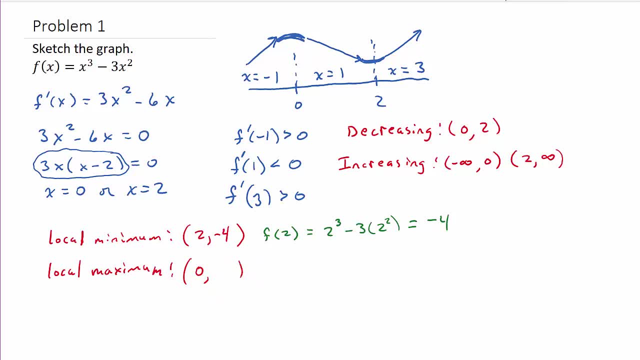 0, and then we need the y-coordinate, so we take the x value and plug it into here. so that's going to be: f of 0 is equal to 0. cube minus 3 times 0 squared and that equals 0. all right, so we're getting there. so we found increasing. 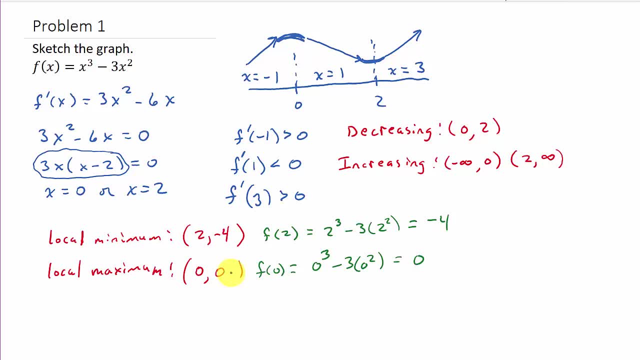 decreasing. we found local max and min. now it's not always going to have a local max and a local mean, and sometimes it might have one or the other. okay, sometimes it may have neither one, all right. so now we've got a fine concavity. we want to know where is the 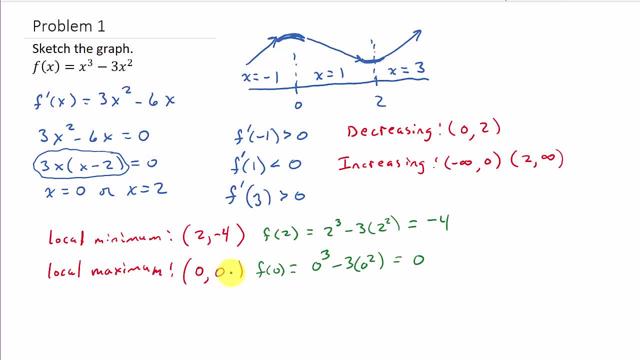 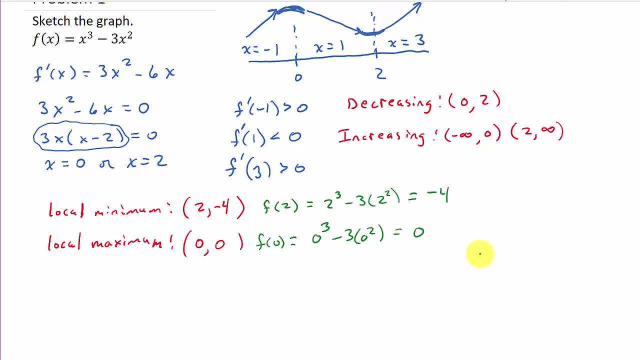 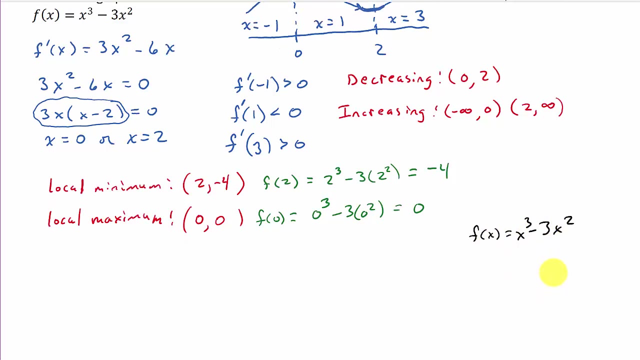 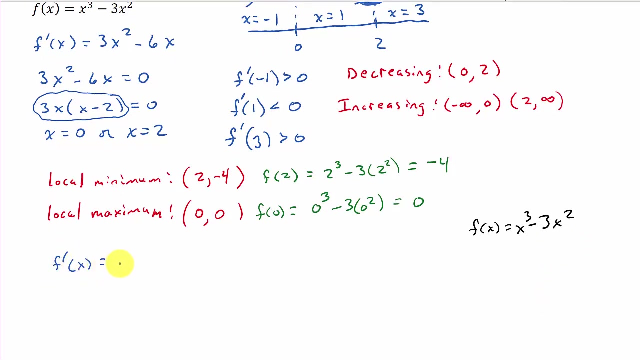 graph: concave up. where is it concave down? all right, so to do that and what I'm gonna do here, I'm gonna go ahead and write my function here, so maybe when we think of something and I say rectify, right now and say rectify. 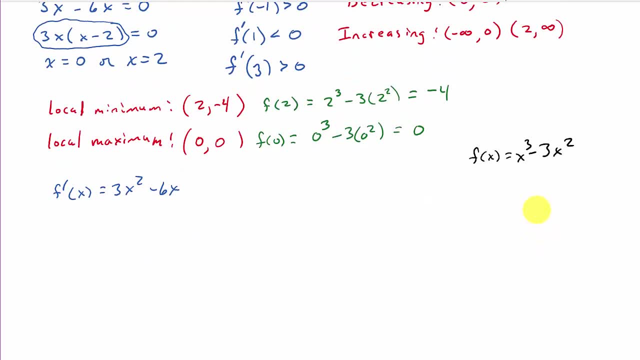 x. Well, I want to opt in a new variable. So now we've got, I'll grid one over, because- and that's going to be 1 up- I'm going to keep that in. now I'm just going to let the y be lounge right, and then I'm going to try and find my function. 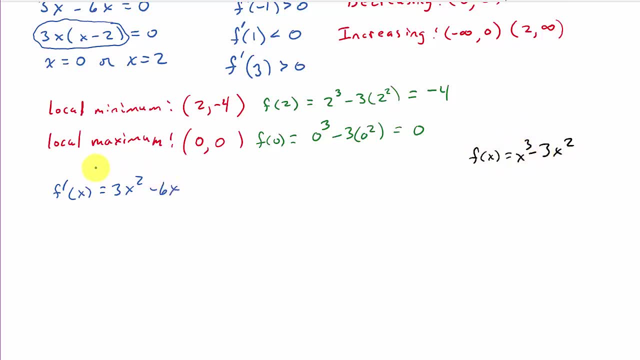 saying 9.0, a very good way to do this. so im going to roll out this on a scale and just of f, of X, which is this, and then we have to take the second derivative, so that's the derivative of this. that's going to be 6x minus 6, and then we set that equal. 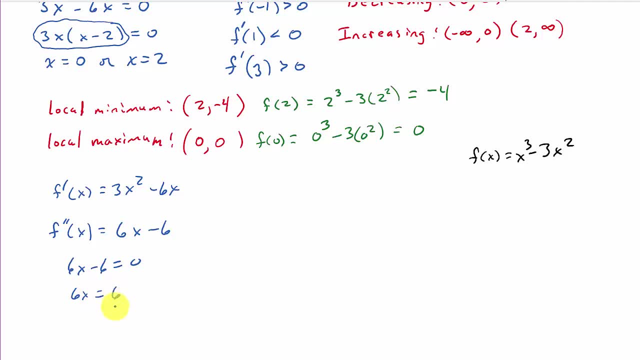 to 0, and so 6x equals 6x equal 1. all right, so now, once again, we draw a number line and plot this value on the number line, and this time we only have one value, so it's only going to break the number line up into two regions and then 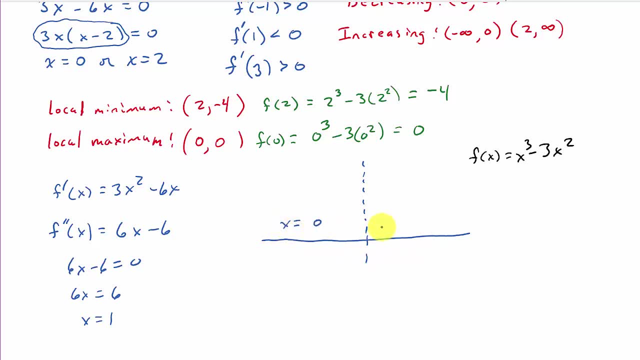 what I have to do is I have to choose a number from each region- makes no difference what values of X you choose, just as long as you choose an X value from each region- and then I have to evaluate the sequence of values from each region, and then I have to evaluate the sequence. 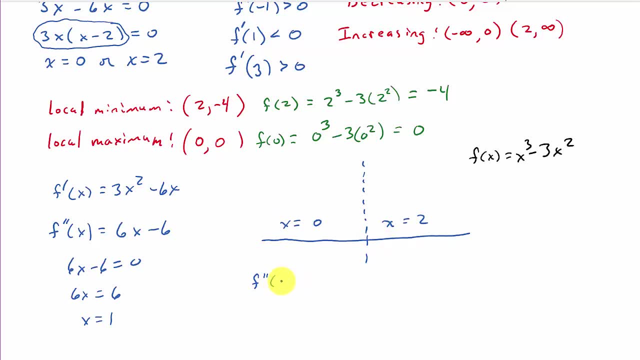 second derivative at each one of these values. so f, double prime of 0. well, let's see, if I plug the 0 into here, that's going to be 0 minus 6, that's negative, so that's less than 0. and since I got a negative value, when I plug the X equals. 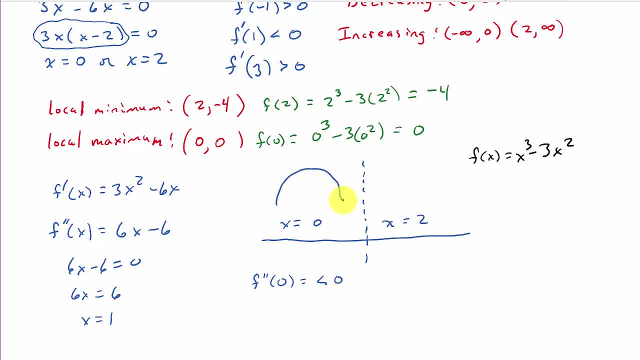 0 in that means on this region it's concave down. and then I plug in the X equal to 6 times 2 is 12, 12 minus 6 is positive and just like before, that's all we care about. is it positive or negative, we don't care about. 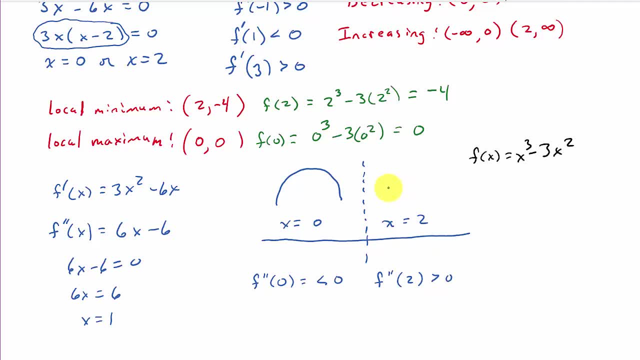 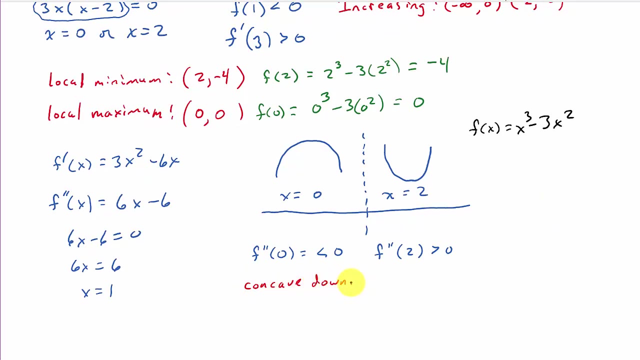 the exact value. so since I got a positive value, that means this is concave up, all right. so now we know that this is concave downward from negative infinity to 1 and concave upward from 1 to infinity, all right. so we found increasing, decreasing local max Min. 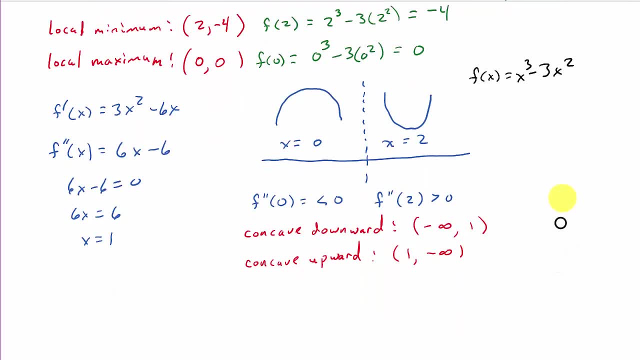 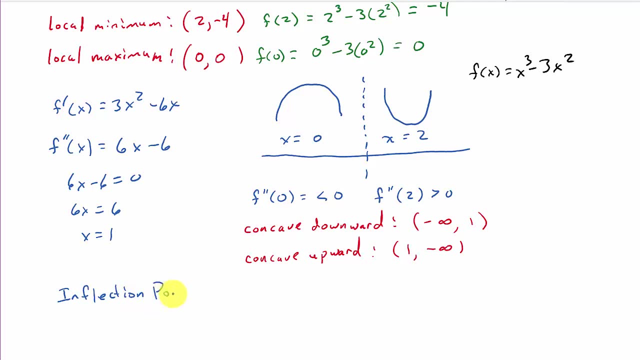 concaved downward the concavity. now we need to find our inflection points. inflection- well, we're only going to have one here, but inflection point, inflection points. sometimes you may have more than one. all right, so the inflection point, that is where the graph 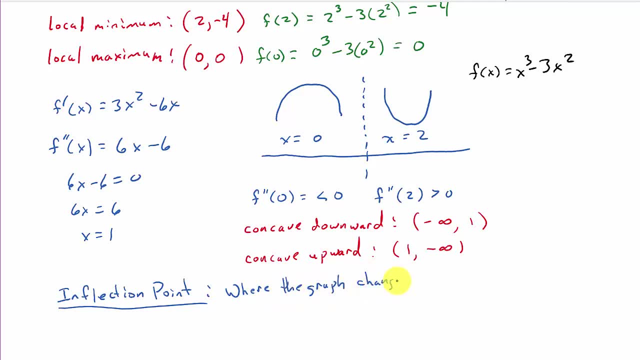 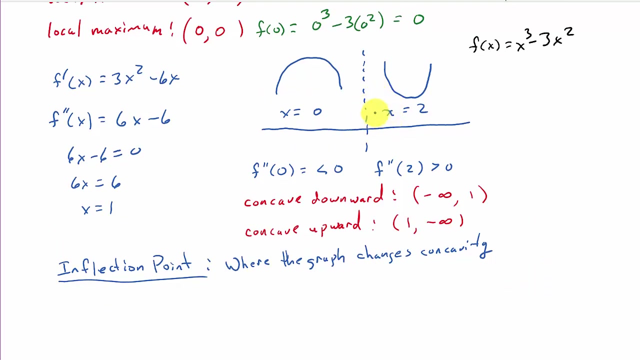 changes concavity. that's the inflection point. so the inflection point that's where it changes from concave down to concave up or concave up to concave down. all right, so we can see here that it changes concavity at x equal one see it changes from concave down. 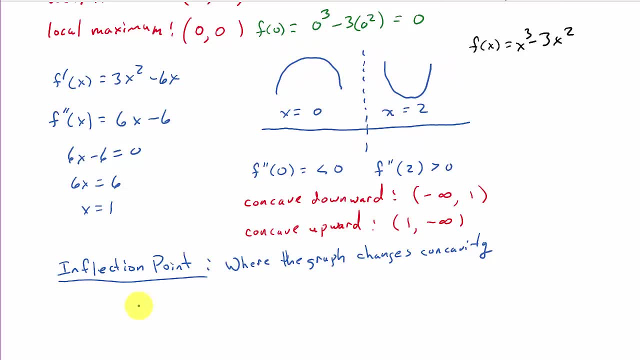 to concave up. so our inflection point is one. all right then, inflection point. it's a point. so we need the x, y coordinate. so we've got the x coordinate and, just like before, how do we find the y coordinate? you plug it back into the original function to get your y value. so that's. 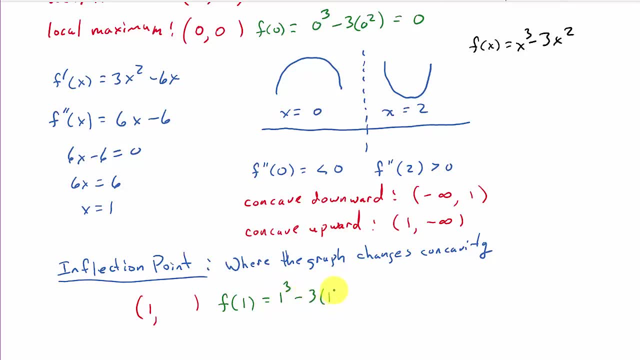 f of 1 is equal to 1 cubed minus 3 times 1 squared, and that is negative 2.. all right, so now we found everything. okay, we found everything. so now we use the stuff that i have written in red, or for you, you know, you put a star by it. 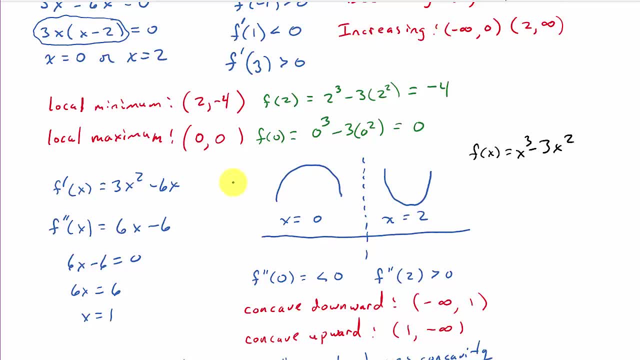 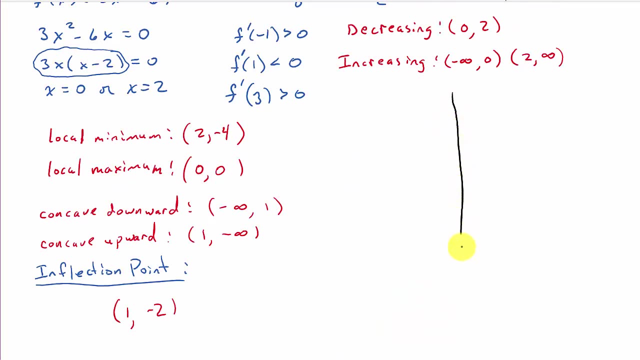 now we're going to use that to graph. so i'm going to erase this stuff and just have all the red stuff on there so we can see everything at one time and sketch the graph, and i'll just pause the video while i do it. all right, so now let's go ahead and graph this thing. so. 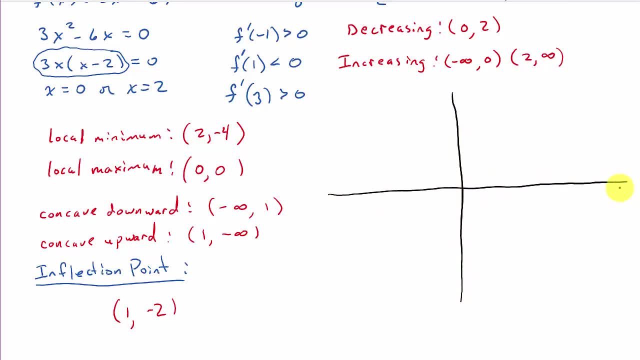 we'll draw us a x- y coordinate system, all right. so let's see, let's look at the points we have. we have two negative, four, zero, zero, and one negative two. so let's do one, two, three, four. one, two, three, four. one, two, three, four, four, all right. so the first thing we want to do let's plot all our points. so we've got the. 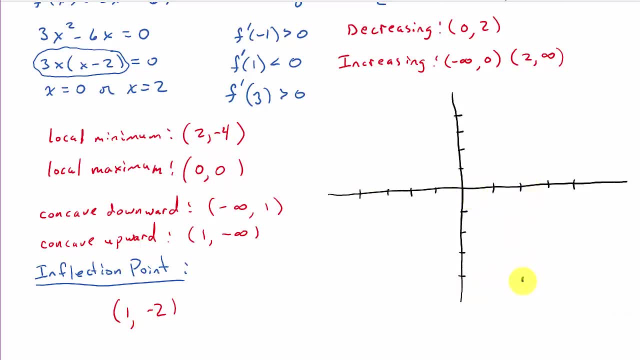 point two: negative four about right in there. one negative, two, zero, zero, all right, so now let's graph it. all right. so first thing I'm gonna look at is: let's look at the increasing and decreasing. all right, so here I've got one, two, three, four, all right so. and then there's 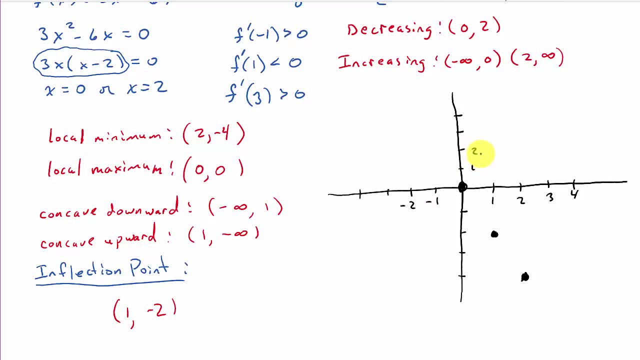 negative one, negative two, so on, all right. so from zero to two, it's decreasing. so that means from here, from X equals zero to X equal to this thing's decreasing. from negative infinity to negative infinity, Infinity to zero, it's increasing. so from negative infinity out here, all the way up to x equals zero. 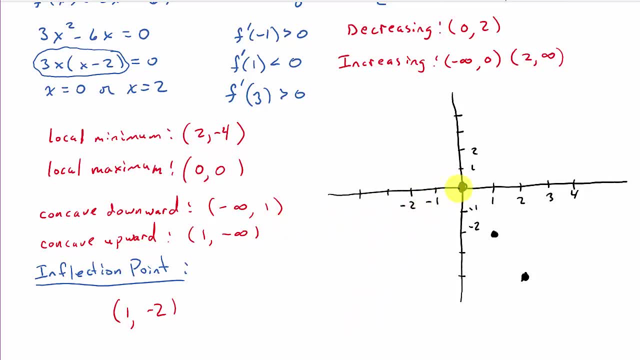 This thing's increasing. you see that it's increasing. So Let's see, that's a maximum at zero. So we've got, let's see, let's draw from here. It's increasing, increasing, increasing. All right, Now you see how I drew this in. did I draw it in right, or should it have been drawn in like this, or?